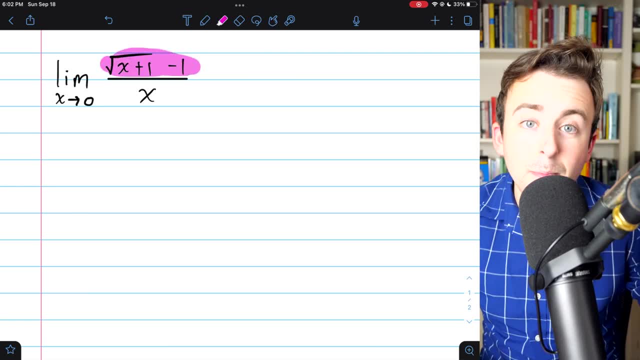 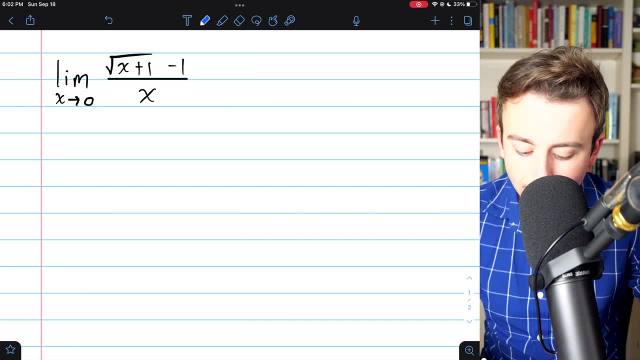 we also have a minus one, So we actually have a binomial here, but this isn't too troublesome to take care of In this situation. in order to rationalize the numerator, all we have to do is multiply by the conjugate of the binomial term that has the radical, The conjugate. 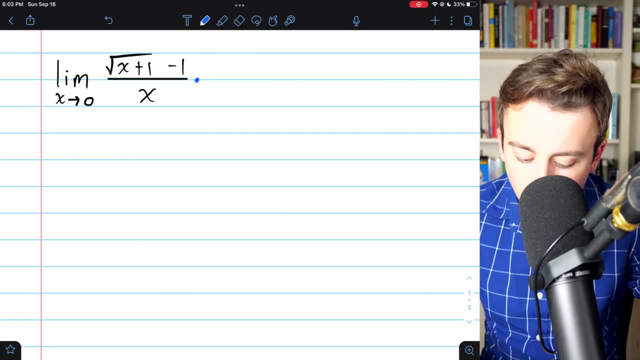 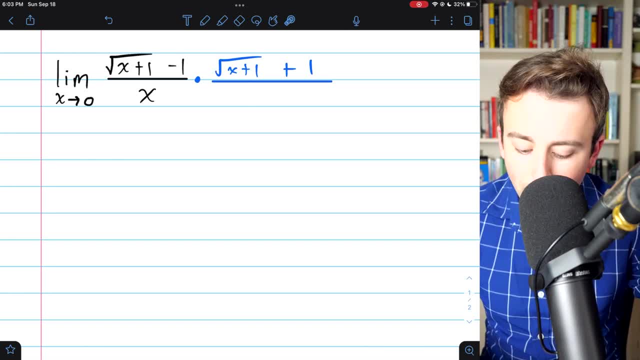 What we're going to end up getting is the square of this thing minus the square of this thing. Now of course we have to multiply by the same thing in the denominator. That way we're just multiplying by one and not changing the value of our limit. So originally we couldn't evaluate this limit by. 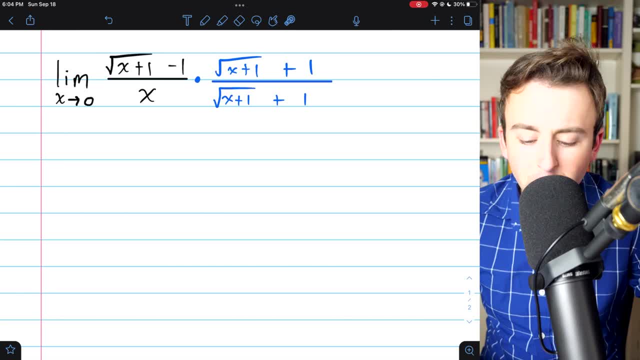 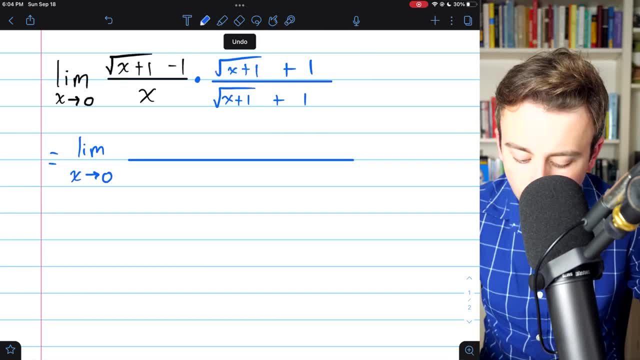 square root of x plus one times square root of x plus one, which is just x plus one. Then we would have square root of x plus one times positive one, and then square root of x plus one times negative one. Those will cancel out, And so the only other term we have in the numerator is: 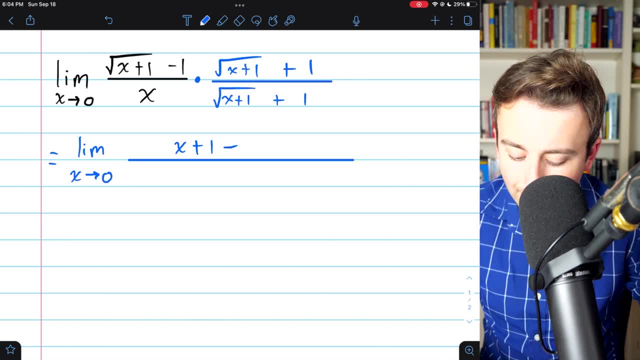 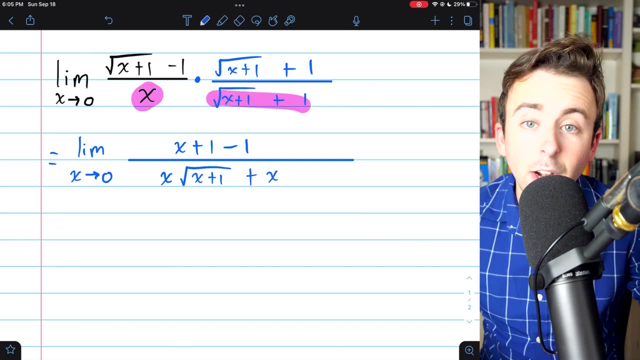 negative one times positive one or minus one. Then in the denominator we have x times the square root of x plus one and then plus x. That's just distributing this x across this binomial. Now in the numerator the plus one and minus one will of course cancel out, And so very. 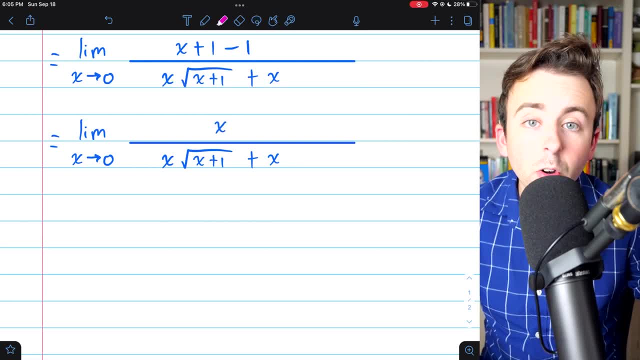 nice, We're just left with x. Now in the denominator we can factor out an x. We've got an x in this term and an x in this term, So at this point we could just cancel out that factor of x. I'll go ahead and just write it to make sure that it's really clear what's going on. 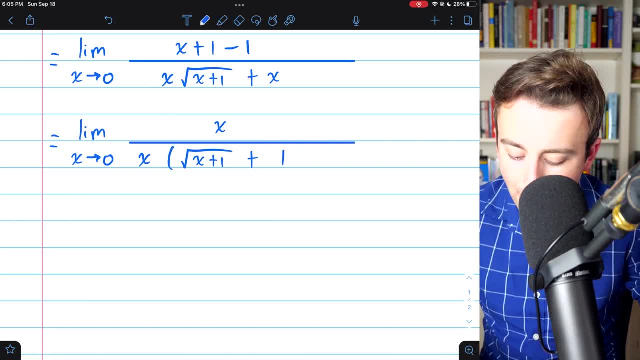 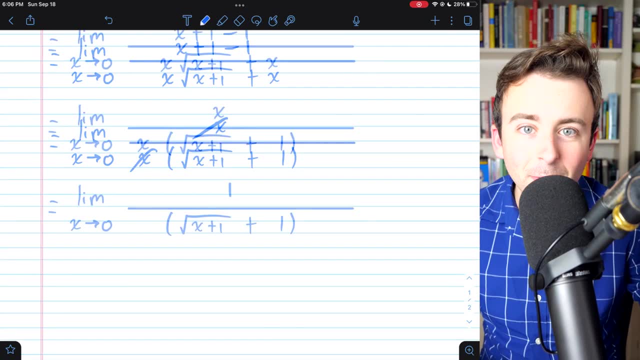 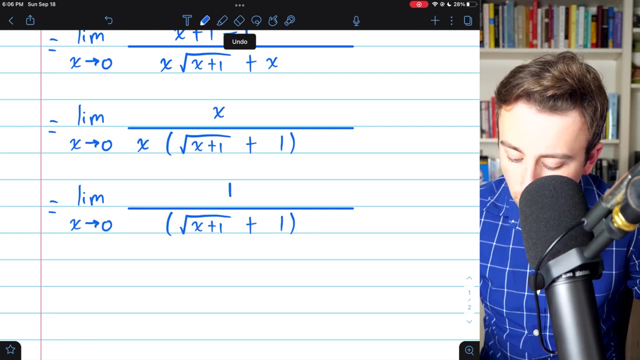 here We're factoring out an x, And so this turns to x multiplied by root, x plus one plus one. And now we can cancel out those x's. And now we've got a limit we can evaluate by substitution. If we just plug x equals zero into this expression, we are going to get one divided by the square root of 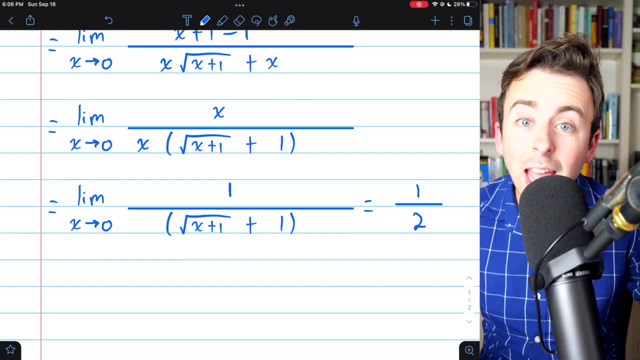 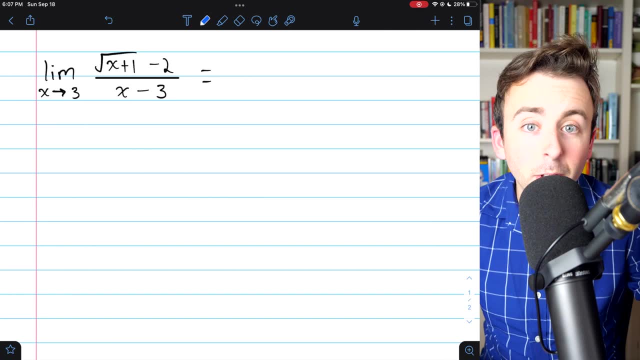 one plus one, or in other words one half. And that's how we can evaluate a limit: by rationalizing the numerator or denominator. Go ahead and give this second example a try yourself. It's a super similar idea. It's just that the factoring we have to do in the denominator is slightly harder to see, but it's very similar. 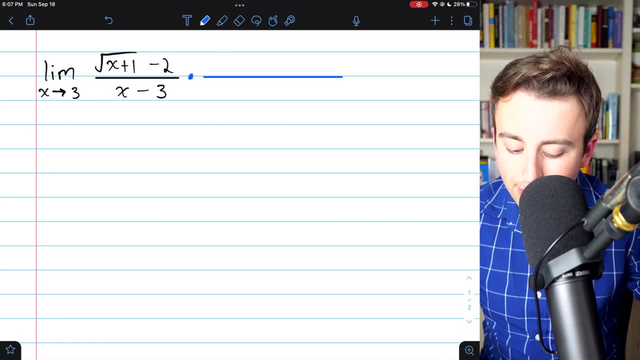 Just as before, the first thing we'll need to do as we attempt to rationalize the numerator in this case is multiply by the conjugate, So that's the square root of x plus one plus two. This is really utilizing a difference of squares, factorization, So we have to multiply by that in. 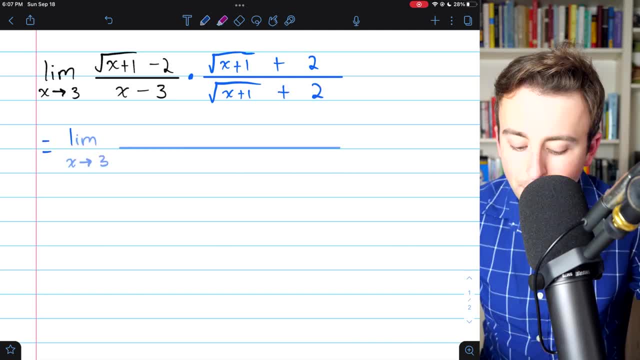 the denominator as well. And let's move on. What do we get? Because this is how a difference of squares is factored. what we'll end up with is just root x plus one times root x plus one, which is x plus one. The only other term we'll have is negative two times positive two, which is minus. 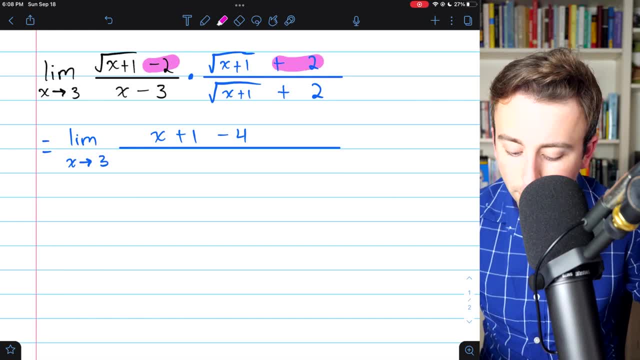 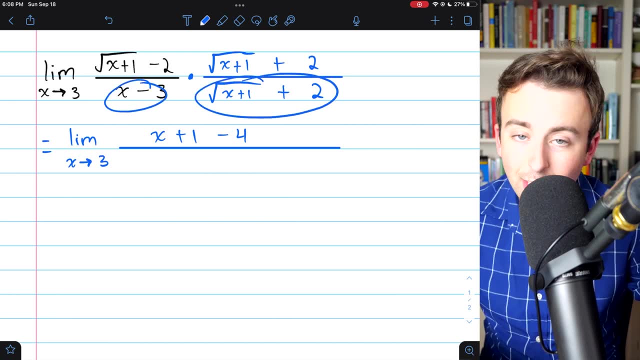 four. The middle two terms, because of the minus two and the plus two, are going to cancel out. And then in the denominator we've got x minus three times this binomial. It might be tempting to do all the multiplication there, but you should notice that in the numerator. 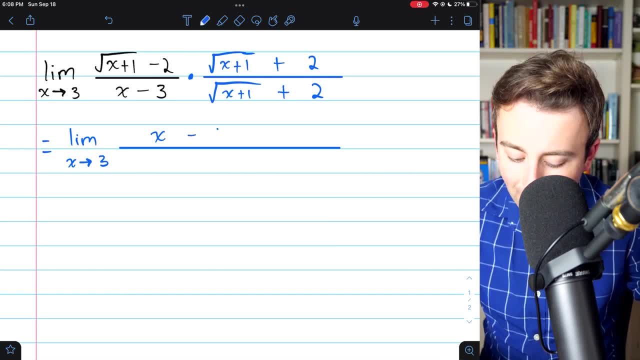 we have x plus one minus four, which is actually just x minus three. So in fact we should probably just leave that x minus three out on its own. So in the denominator we have x minus three, times the square root of x plus one plus two, And I guess I don't know what. 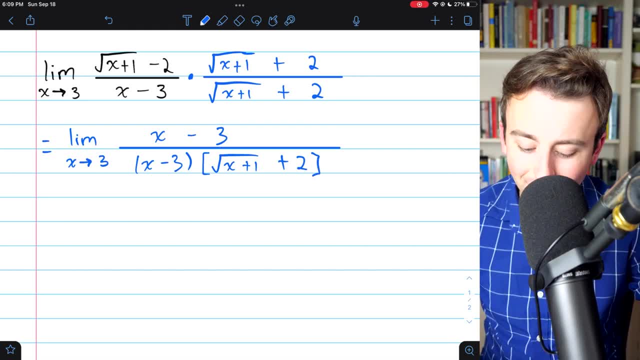 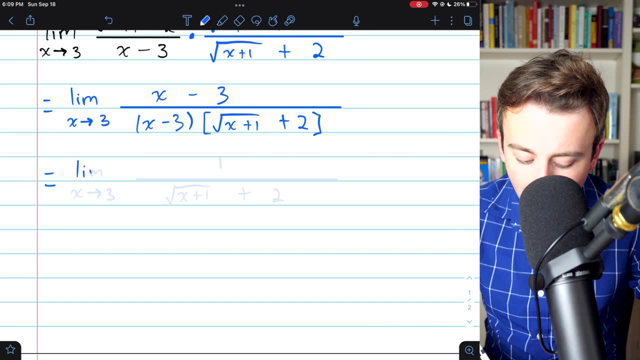 I was talking about saying that this one was harder. It's pretty much exactly the same as far as the mechanics go. So then what will we do? We'll cancel out the x minus threes, and then we're pretty much done. At this stage we can.